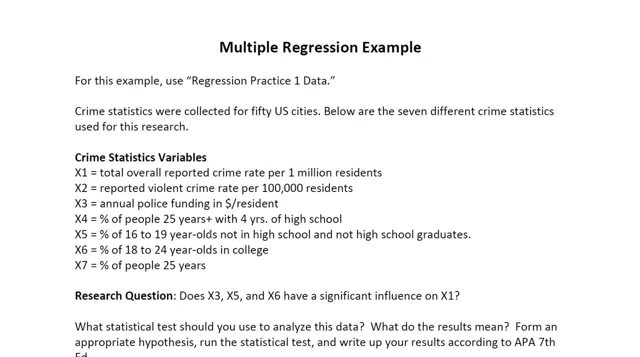 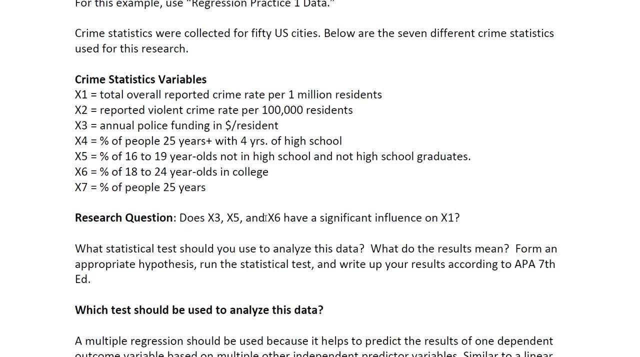 collected from the 50 US states and here are the variables. Now the difference is our research question. So in this case we're looking at if x3,, x5, and x6, so 3,, 5, and 6 up here have a. 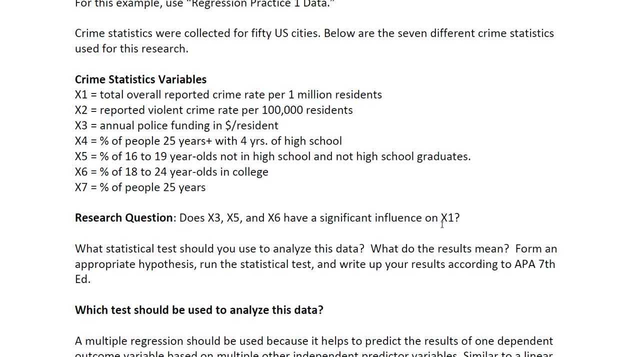 significant influence on x1, which is the total overall reported crime rate. So, basically, what we're trying to figure out is if these three predictor variables- these are our independent response predictor variables- have a significant influence on our outcome. slash dependent variable of x1.. 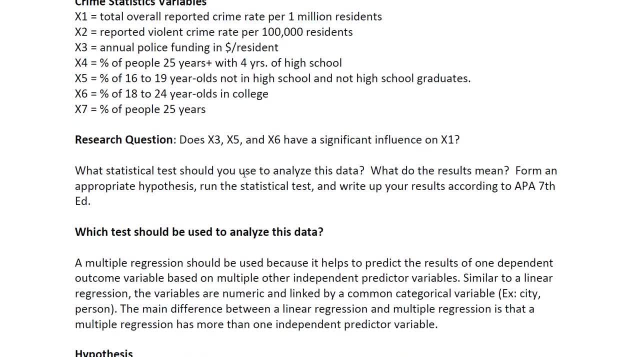 So the questions we're thinking about are: which statistical test should you use to analyze this data? what do the results mean, form an appropriate hypothesis from the test and write up your results according to APA 7th edition. So for which test a multiple regression should be used, because 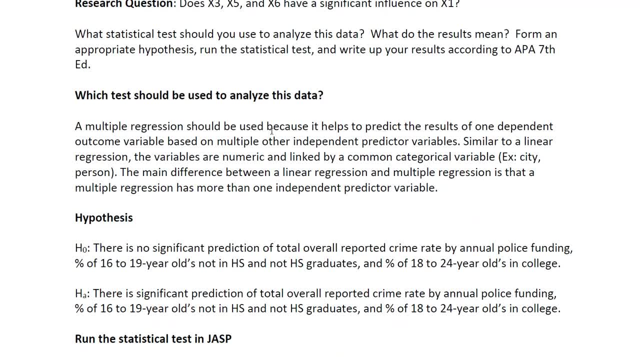 it helps predict the results of one dependent outcome variable based on multiple other independent predictor variables. It is similar to a linear regression and the variables are numeric and linked by a common categorical variable. In this case it's city, but it could be a person, it could be schools, so individual schools it could be. 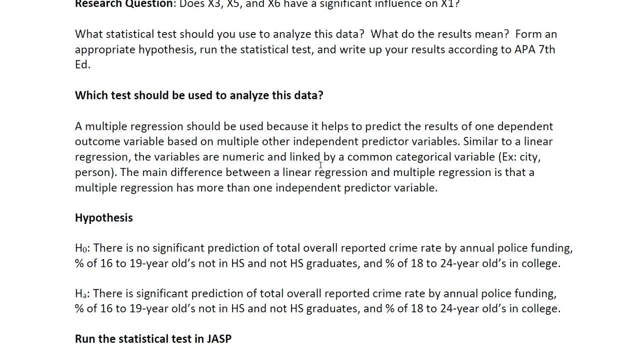 individual businesses. There's lots of different things that could be that common categorical variable, but they have to have one. That's the important part. The main difference between a linear regression and a multiple regression is that a multiple regression has more than one independent predictor variable. Otherwise, you're going to see that they're pretty similar. 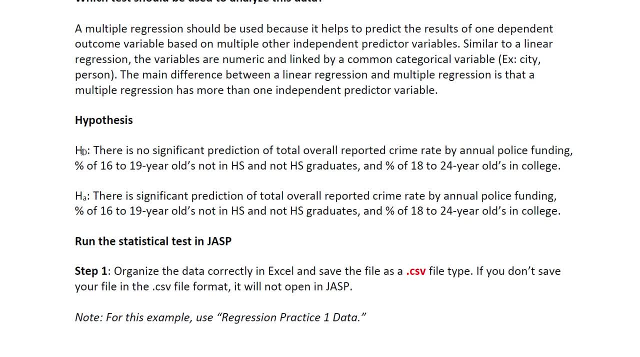 So for our hypothesis, our null hypothesis, is that there is no significant prediction of total overall reported crime rate by annual police funding, Percentage of 16 to 19 year olds not in high school and not high school graduates, and percentage of 18 to 24 year olds in college. 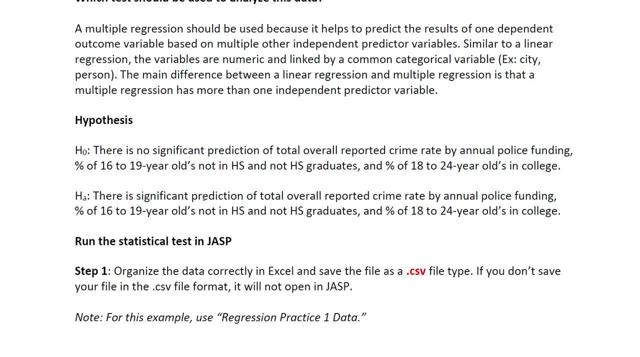 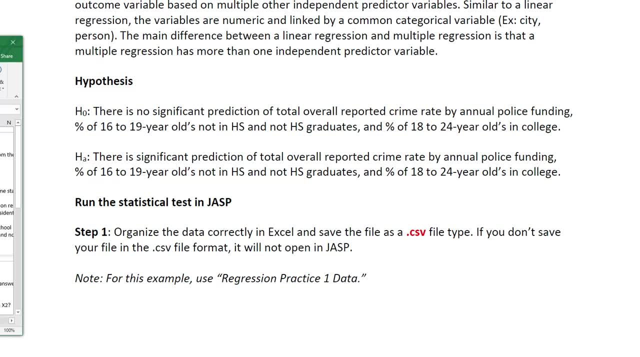 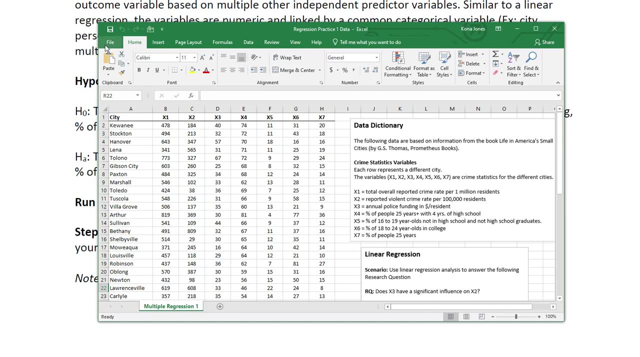 Our alternative is just that there is a significant prediction. So next up is running the Statistical Test in JASP. So remember, here it is right here. Here's that data and the. And the first thing we need to do, if you haven't already, is we need to save it as 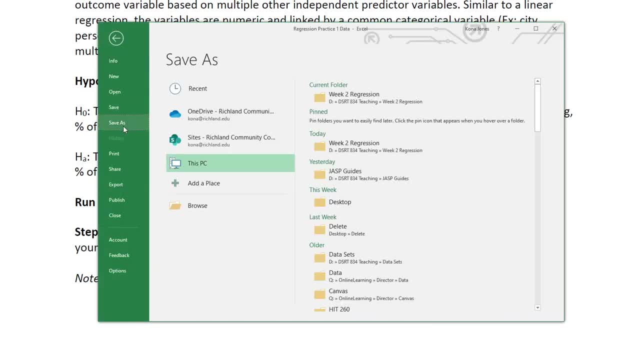 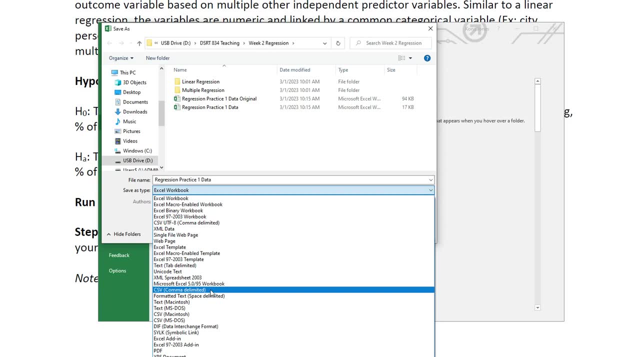 a CSV file. So we're just going to go to File Save As and I'm going to pick this folder. but you can pick whichever folder you want, then come down here and we want to save it as a CSV, comma delimited. 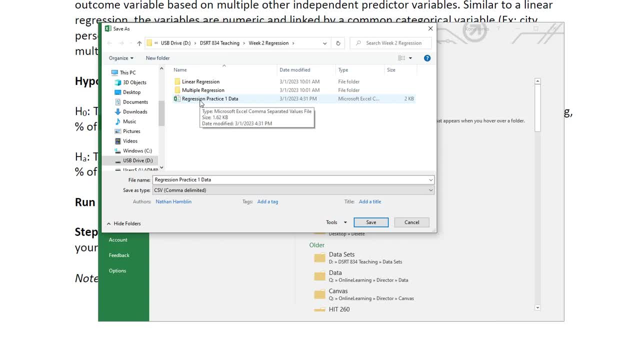 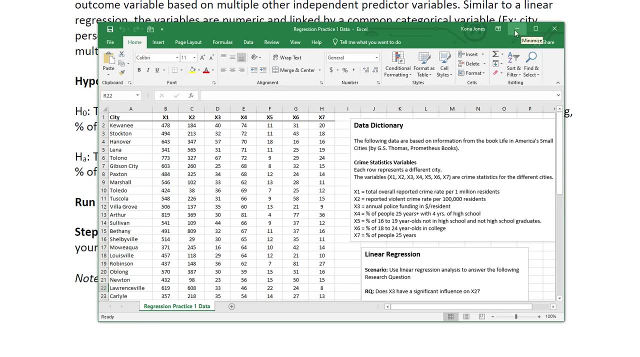 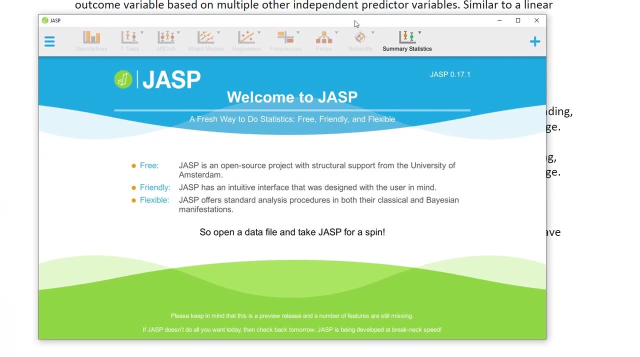 In this case. you can see, I do already have it saved like that. so if you do, that's fine. You don't have to re-save it, otherwise, just go ahead and re-save it. Okay, so now that we have that, we can go ahead and get rid of this and move into JASP. 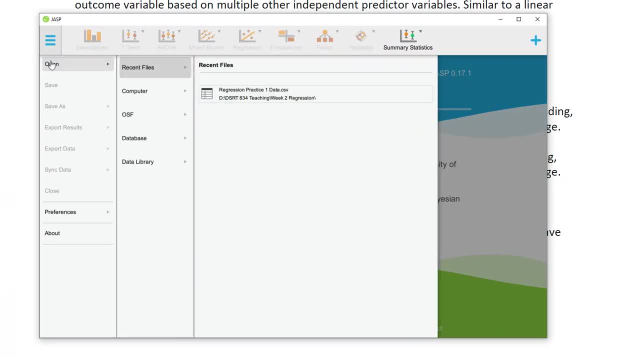 So to open that file. we're just going to come up here to that main menu. go to Open If it's a recent file. so if you used it for that linear regression example it might already be showing up here. Otherwise you can go to Computer Browse. or in this case, mine is right. here it's. 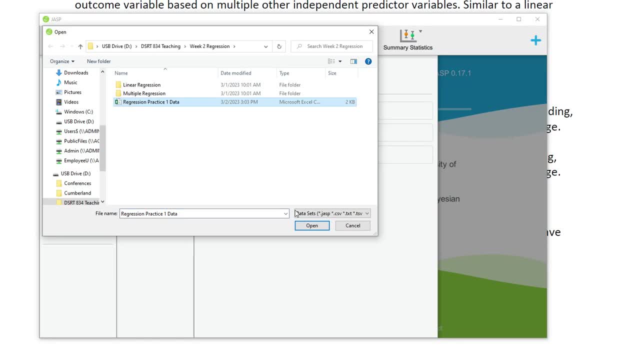 my Week 2 Regression and I can just go ahead and click on it and click Open. So now, once it opens up, we're going to go ahead and save it as a CSV file. So now, once it opens up, we're going to go ahead and save it as a CSV file. 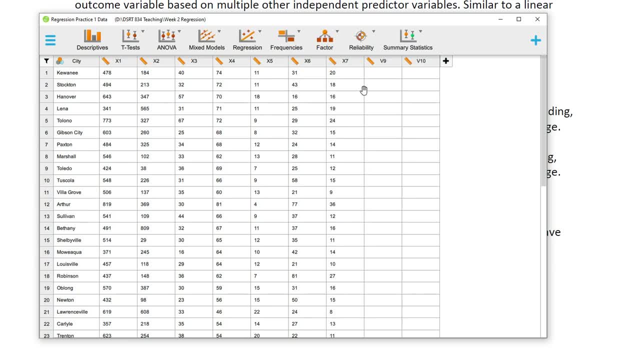 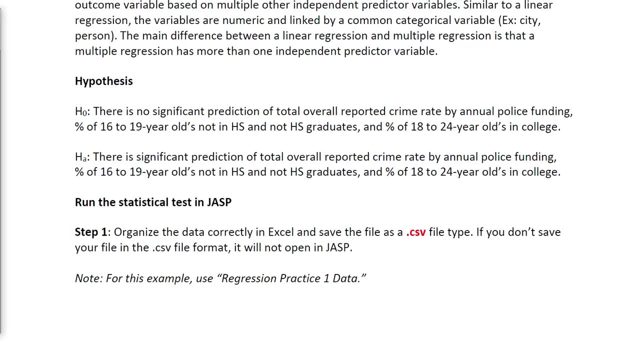 So now, once it opens the important thing: Ah, we've got some extra variables hanging out there. I'm not sure why those are hanging out there. Don't worry about it. If you wanted to clear them out, So hold on, I'm going to show you how you can clear it out, if that bothers you. 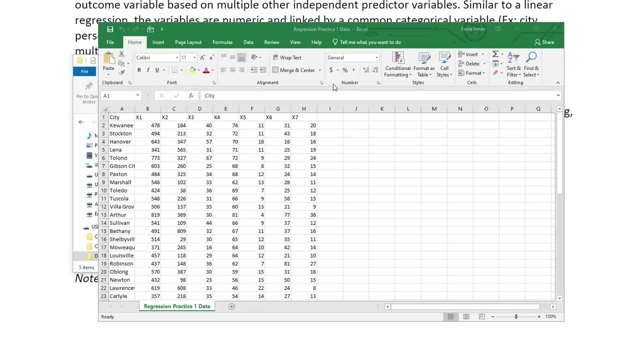 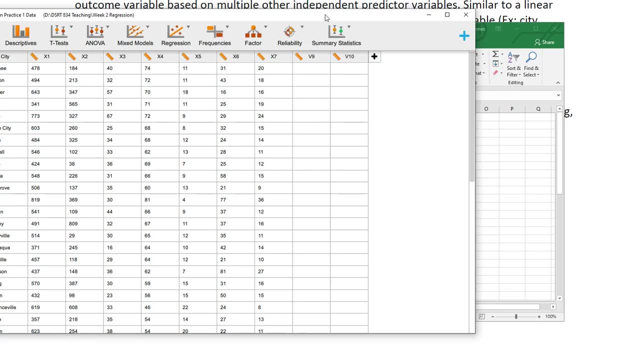 Okay, So I pulled up and this is the CSV file. So I pulled up the CSV file and what this JASP file is showing is that in these two columns it thinks there is something there And it's probably because of those boxes of information. 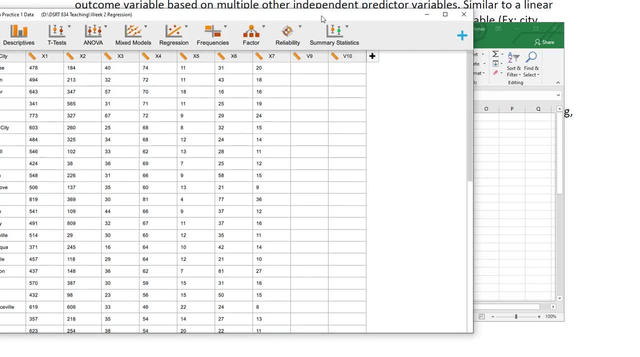 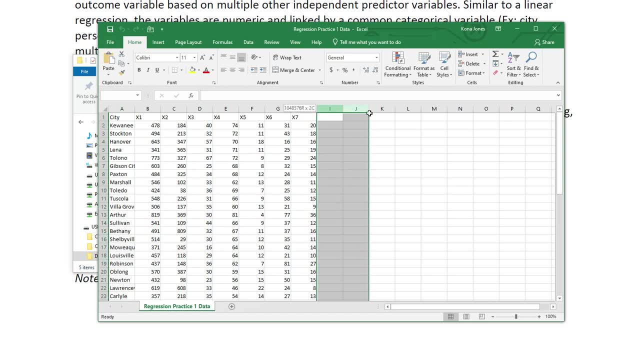 dictionary that I had in the regular file. that's probably what's kind of given it fits. so all you need to do over here is just come over and you can pick as far out as you want, and then right here it's going to clear out the data. so 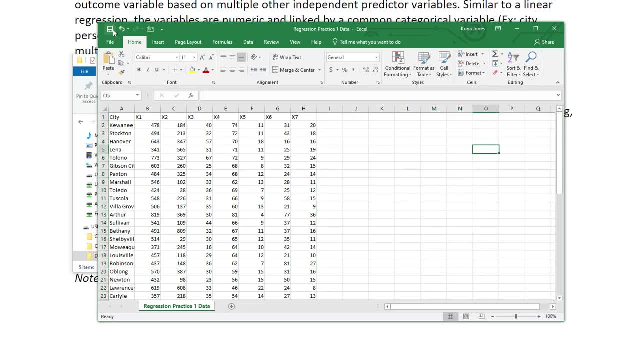 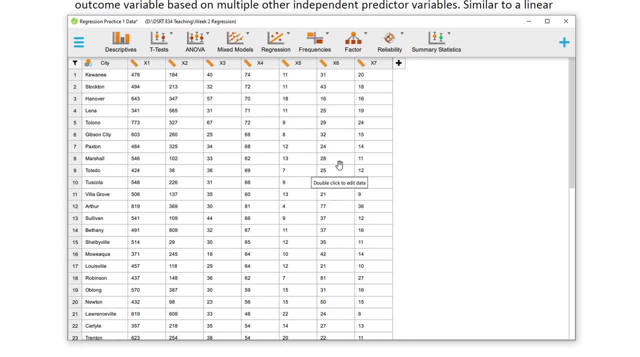 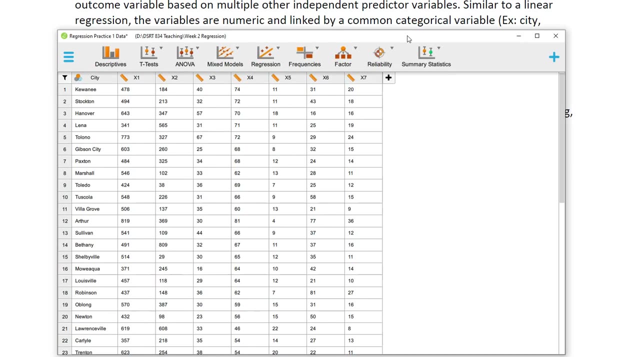 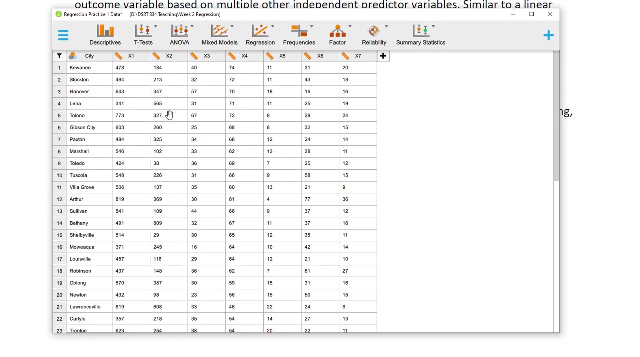 clear all. I'm just gonna clear all- and then click Save and then remember the magic of JASP, because they are linked. JASP is going to go ahead and automatically update, and now those two columns are gone. okay, so here we are, in JASP, and now what we're going to do is, first of all, make sure that all of these 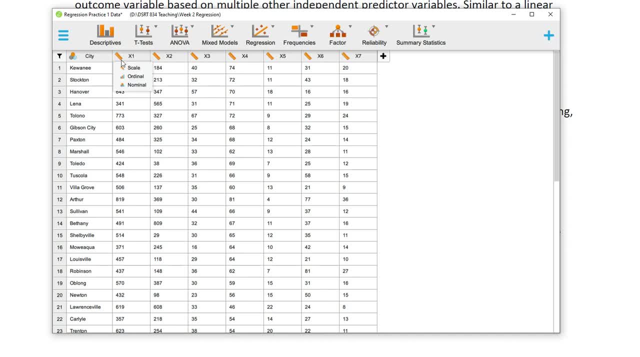 variables right here, the ones we're using for the regression, that they are scale data. if they were ordinal or nominal, that would not work. they need to be scale. we will have this first one right up here, right, that's nominal or archaic categorical variable and those are just the cities for each of these rows of. 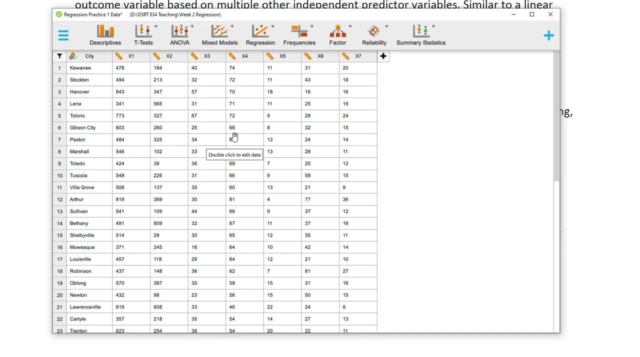 data. now for the actual multiple regression. it's going to look really similar to what we did for the linear regression: we're going to come up to regression and instead of correlation or linear regression- oh wait, a second- we are, and this is why we say multiple regression and linear regression are so. 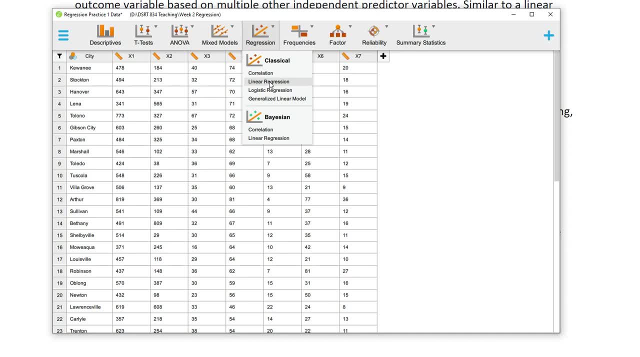 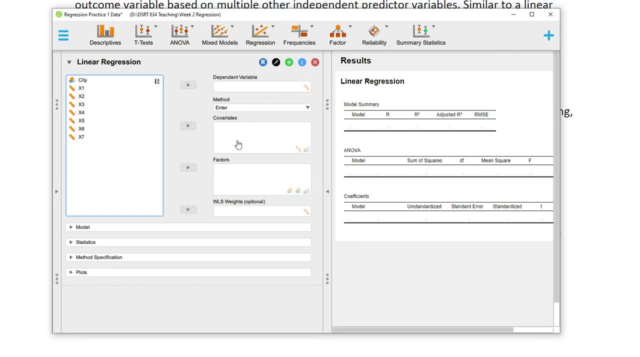 close is that little linear regression is going to be what we use for the multiple regression. so, when we pull this up, the only difference is going to be that, instead of just having one covariate, one independent variable, we will have the three covariates. so we'll start with our dependent variable or our 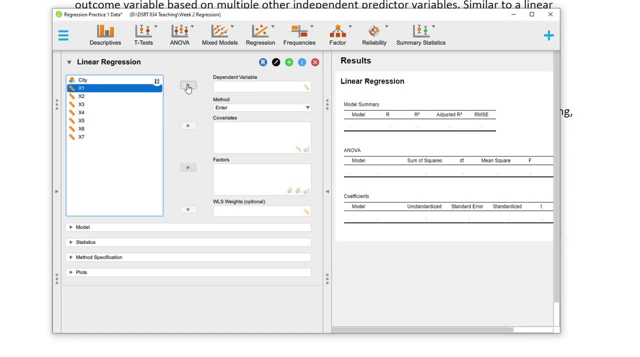 outcome variable, which was x1. so remember, that's the thing we're measuring, that's the thing we're trying to predict, that's our outcome, our dependent variable, and then we're going to go ahead and put in our covariates. now, these are going to be our independent variables, our predictor. 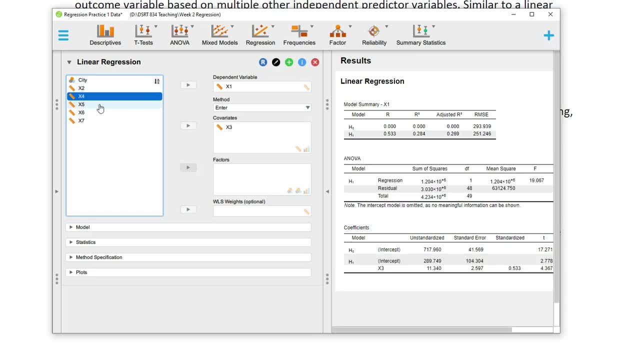 variables, and so in this case, we have our x3, 5 and 6, so we've got a love jazz, because it just automatically, right, starts tabulating things for us. the only thing we need to do now is underneath statistics. so pull that one down, make. 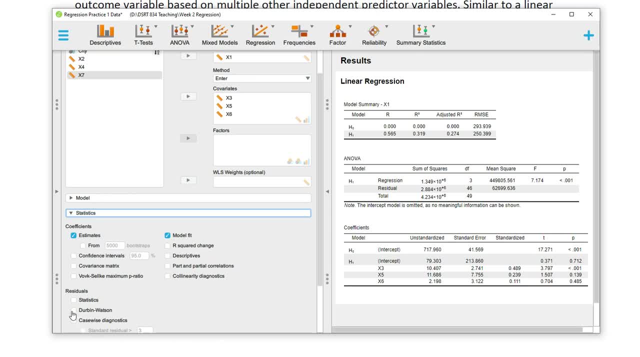 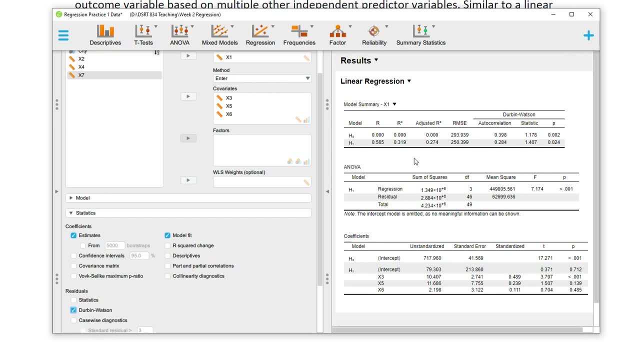 sure you have estimates, make sure you have model fit and then just add in underneath residuals the Durbin box and that is all of the data you need for the multiple regression. so now, as we go through and interpret it, let's go ahead and start with our first box. so, unlike 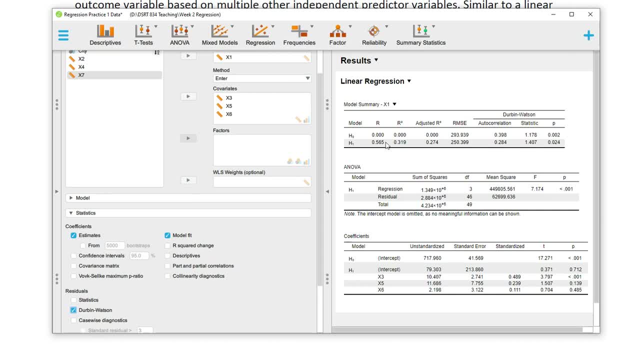 the linear regression of the correlation. we're not going to look at the R value and we're not going to look at the R squared value. instead, we're going to look at the adjusted R squared value and specifically the h1. so the alternative, this is what we are actually testing and so, in this case, our adjusted R squared. 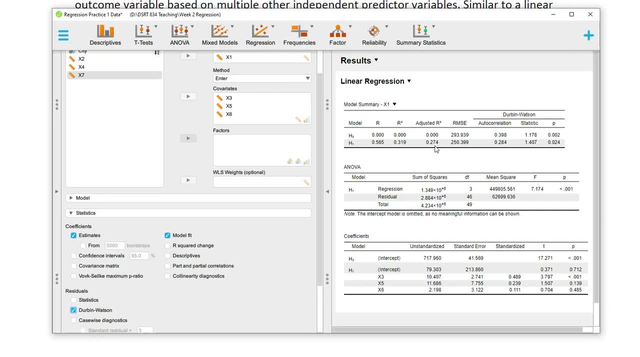 variable variable is 0.274. now, remember that it's going to be similar to our R squared in terms of how we explain it. so this is just going to be the variance that is explained in our outcome variable when you factor in your predictor variables. so, similar to. 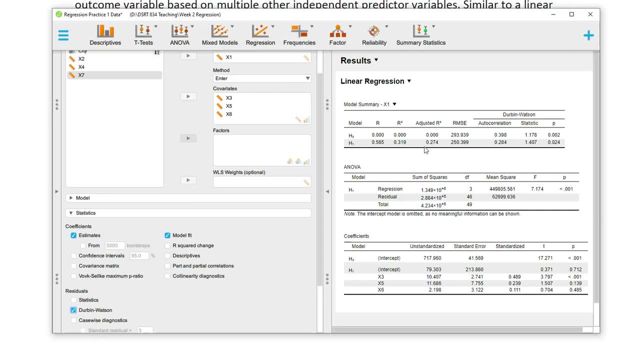 last time. this is a fair right. this is so a fair amount of the variance is explained. so a fair amount of the variance in the total prime rate is explained by our three predictors, but not by this one. so we're going to go ahead and too much. Now. the reason that we're using our adjusted r instead of our r squared is that we 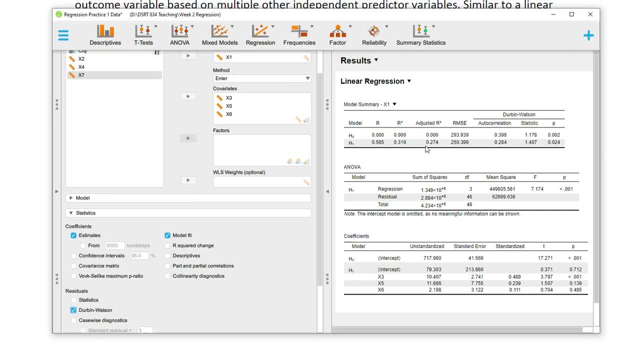 have more than one independent predictor variable. So when there was just one independent predictor in the linear regression, we used r squared. But since we've got more than one independent predictor variable- in this case we have three- we have to use that adjusted r squared because 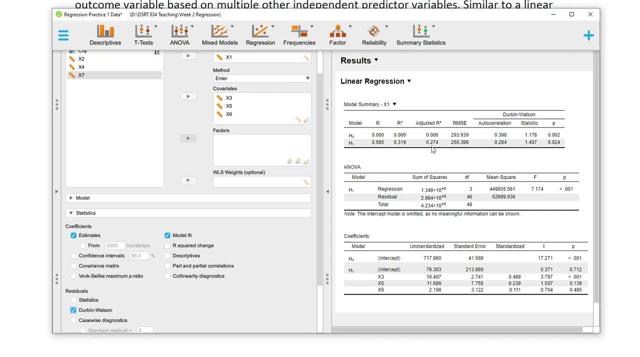 what that adjusted r squared is doing is that it's going ahead and taking into account the residuals of all of the variables, not just the residuals from the r squared variable. The other one that we need to look at on this one is that Durbin-Watson And so remember. 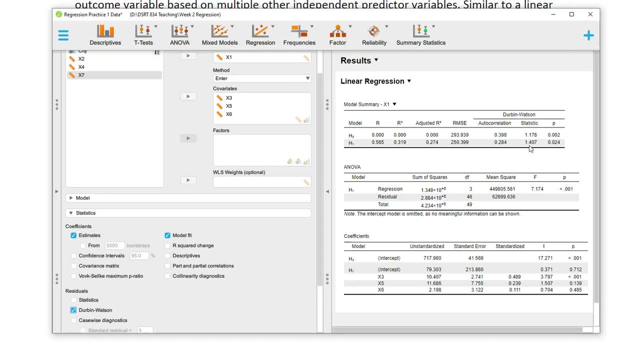 we don't look at anything on that top line, we only look at the second line. So it's the 1.407 is the Durbin-Watson value For this one. we want it to be higher than one and lower than three. 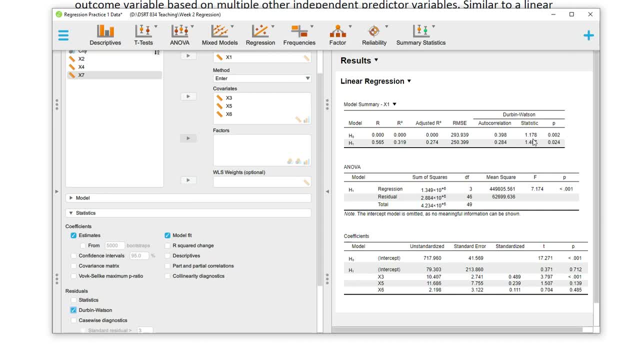 which it absolutely is. So that means that this data is good to go. we can use it. So, moving down um, the ANOVA table is the one that's going to give us our actual multiple regression like outcome. This is the p-value right. This is the important p-value right here is on this ANOVA. 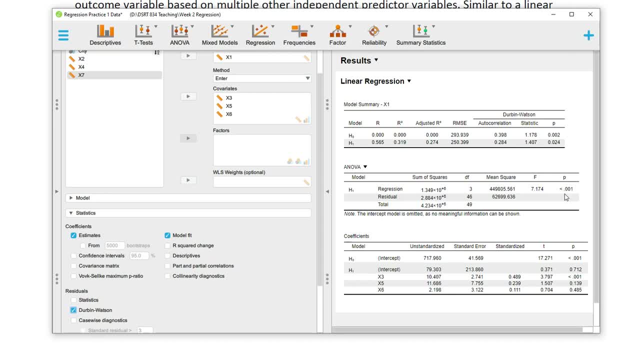 table And this p-value is much less than 0.05, which means that it is a significant right. So our results are significant. It is a significant prediction going on of our three predictors for the outcome variable. It also means that we will reject the null because our p-value 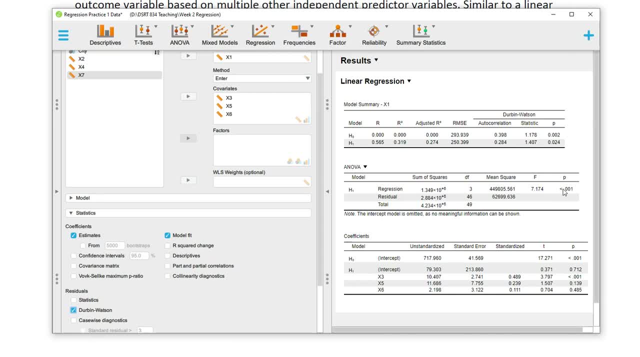 is low, So we are rejecting the null. The other value that you're going to want is this f-value, right here, So it'd be our f-value, the p-value, and then for degrees of freedom, So, similar to the linear regression, you're going to use the regression: degrees of freedom and the residual. 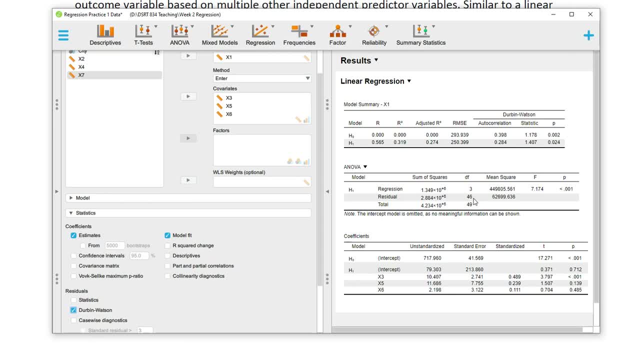 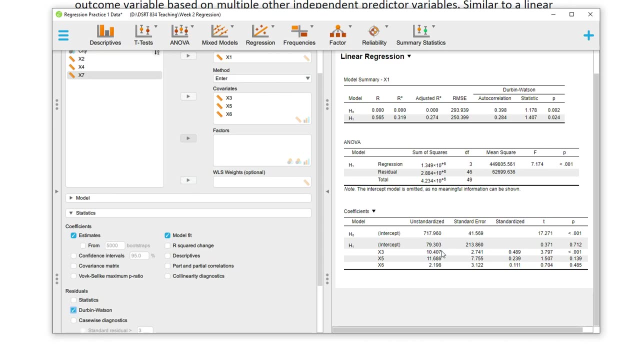 degrees of freedom. So the degrees of freedoms would be parentheses three, comma 46.. That's the degrees of freedom. So our f-value- degrees of freedom- and then our p-value. So the last one is this: coefficient. And for the coefficient, what we're looking at once again, 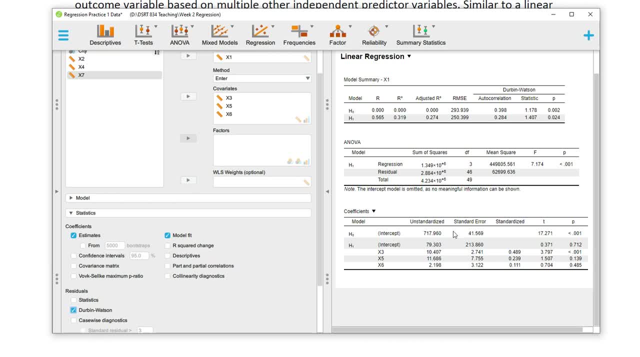 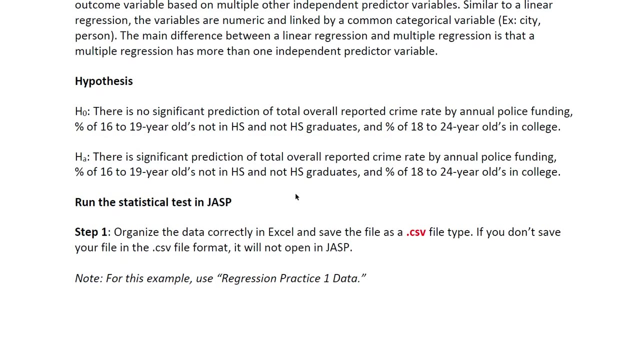 we don't look at anything for that, for the null, for the H0 model. Instead, we're only looking at the H1 information. So the information here that we need is the intercept, the x3 coefficient, x5, and the x6.. Now I'm going to switch over to here- We don't need this one anymore- And scroll down. 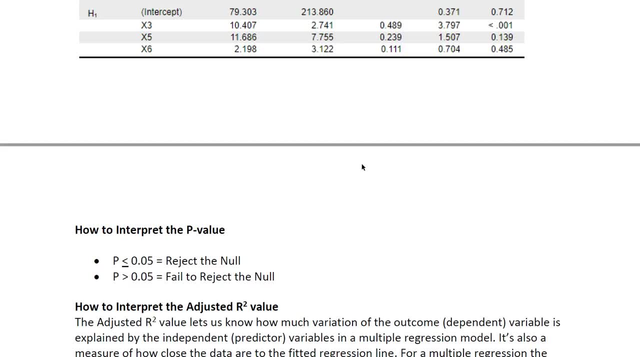 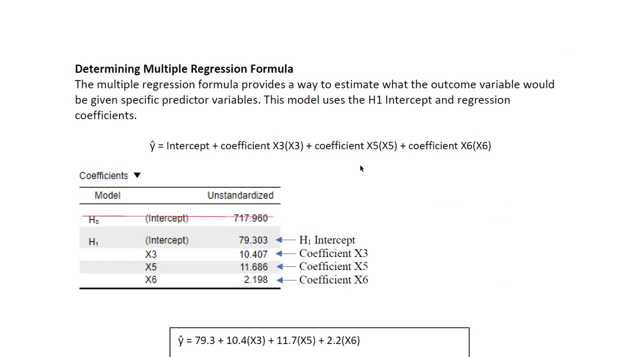 So I explain everything that is talked about on here So you can- hopefully you're taking notes And all of that- And here we go. So you can see. the multiple regression formula is similar to the linear regression. The only difference is that you are adding more coefficients, So instead of just 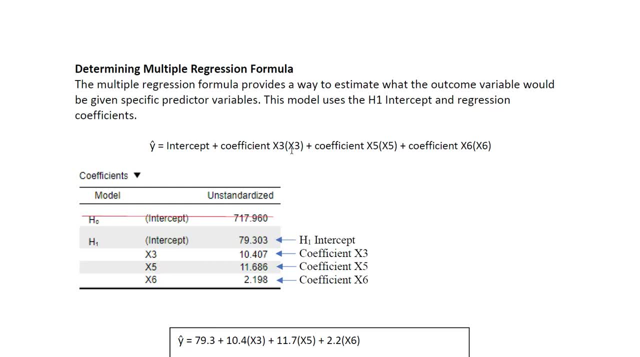 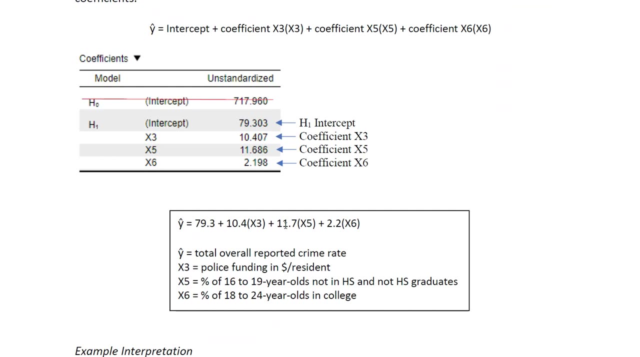 one coefficient. you now have the three coefficients. They are multiplied by the value. So whatever that value is, that would be the thing in the parentheses for each one, And I know that might not make sense, So I do have down here what the formula looks like as well. as you know, the y-hat is just. 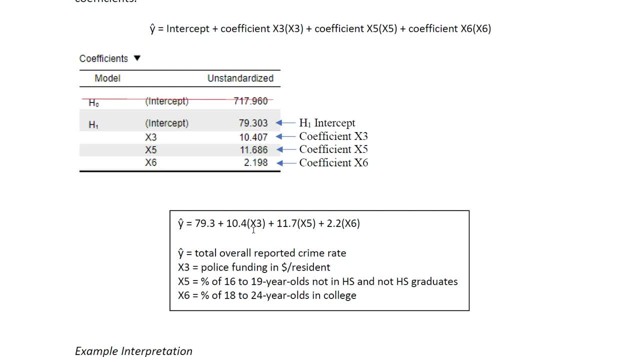 our total overall reported crime rate x3, you know, that's the x3 value that would go there, x5 value would go there And x6 value would go there to give you what y-hat is. So an example of this, and this is kind of similar once again to linear regression: 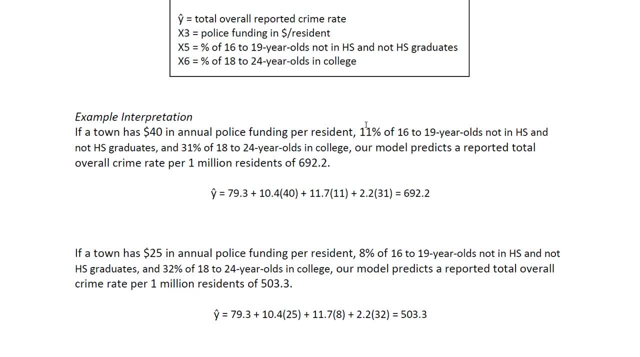 So I had the $40 in annual police funding, but then I added 11% for the 16 to nitrate, 6% for the 22 year olds And 31% for the 18 to 24 year olds. So when you plug that into the 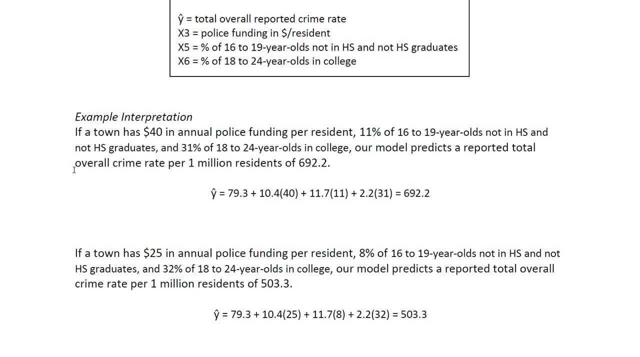 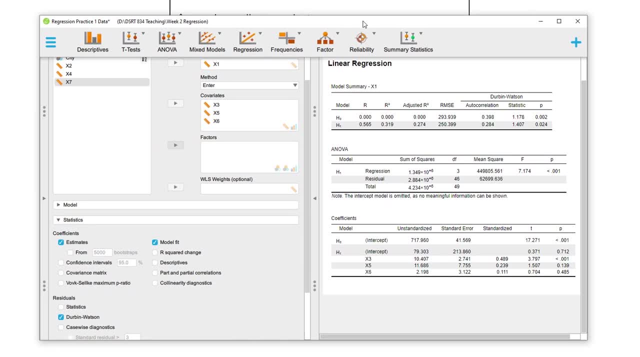 formula: your 40,, your 11,, your 31,, you get 692.. As the overall crime rate for 1 million residents. So the interesting thing, though, is, if we come back over here and let me just go ahead and get out of, 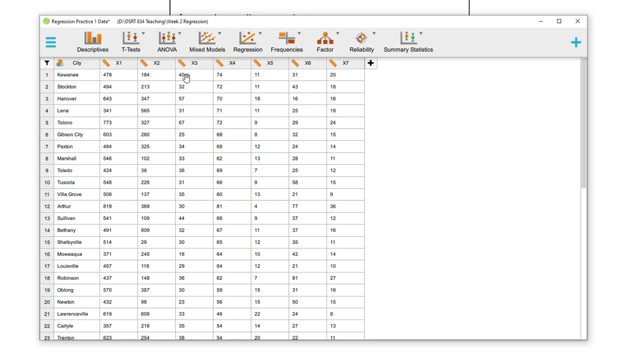 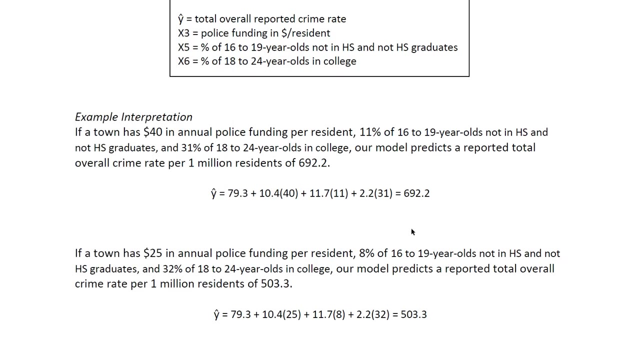 here is that. here is an example of where I got that data. So I use this 40 Kiwani and then I used the 11 and the 31.. Well, this is the actual. so their actual total overall crime rate was 478, yet we're estimating that it's 692.2.. That is not even remotely close right. 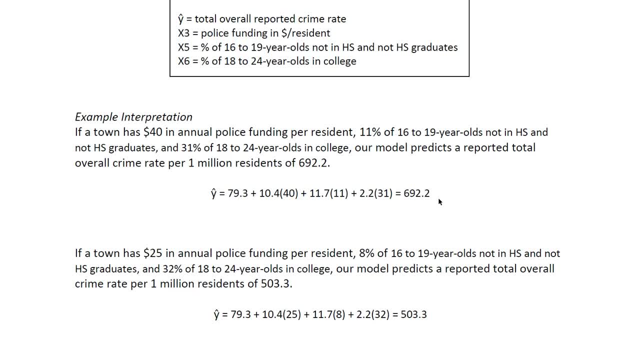 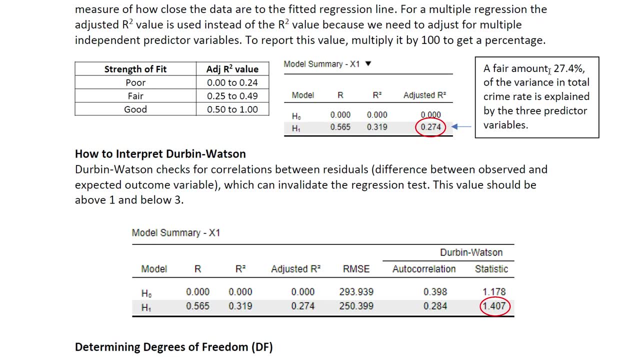 So this is where that R-squared adjusted comes into play, and the fact that it was only 27.4.. So remember, only a fair amount of the variance in total crime rate is explained by the three predictors. So this is why that value is kind of so far off, is that? well, why? but the 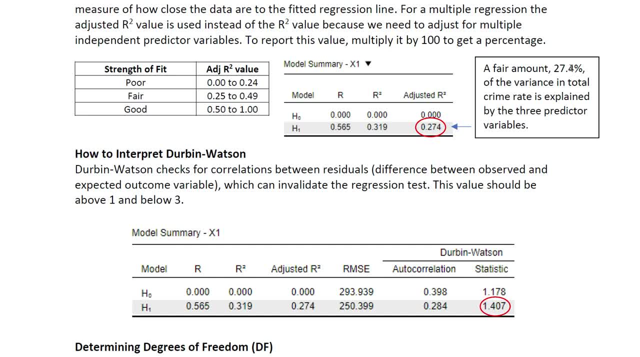 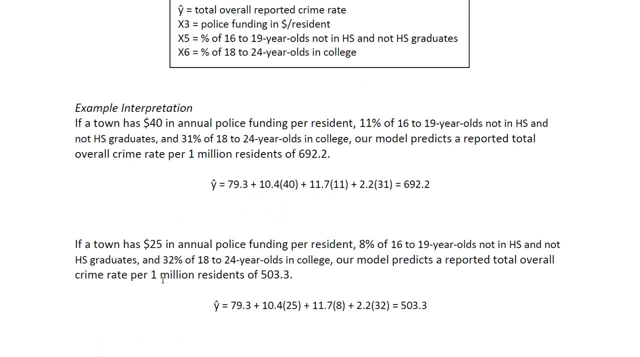 why it is is why this is kind of so small and that it's not explaining more variance. is that our model, while it is significant, is only explaining a fair amount of that variance. It's not doing a amazing job by any stretch of the imagination. Yet if you come down and you look at this, 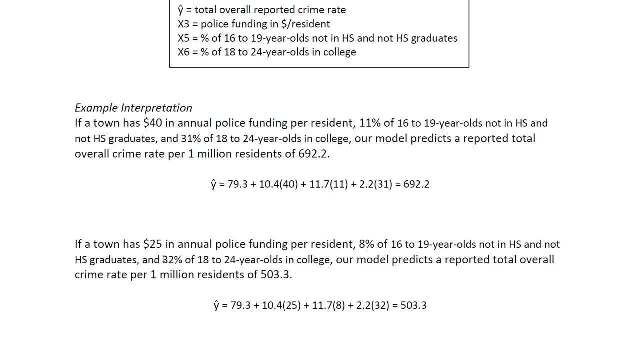 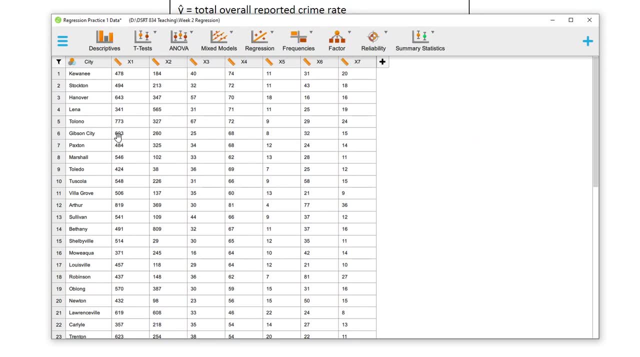 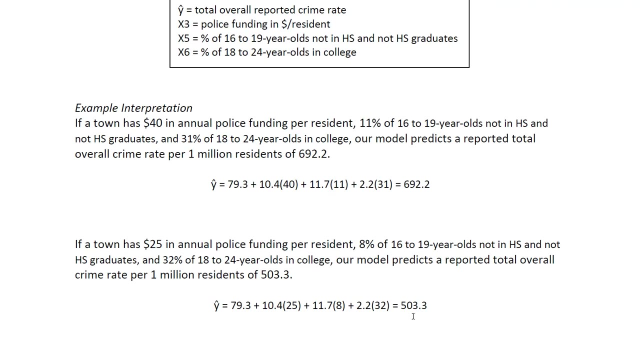 example. so the 25 and 8% and the 32%, and that's this one right here. so 25, 8, and 32, you can see their overall total crime rate is 603, which is compared to 503.. So that's only 100 off, which is 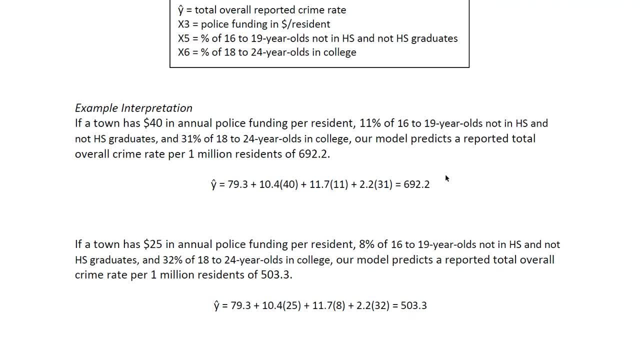 a lot closer. So this is where, like, this one might be quite a ways off, but this one might be pretty close. And that's why it is significant, because I mean I bet if we went and we ran all of. 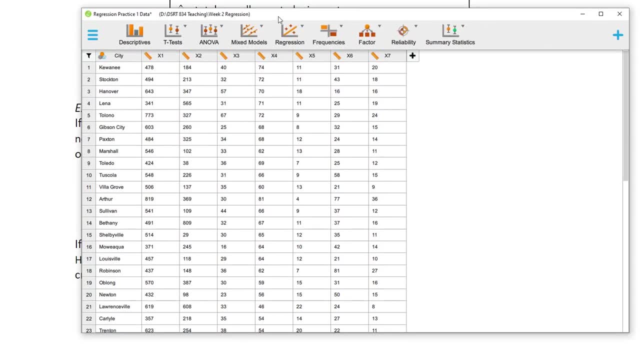 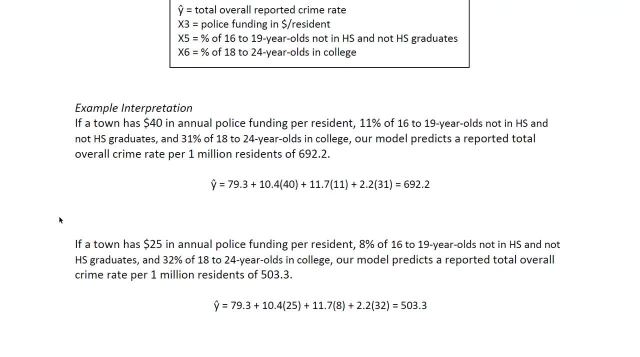 these to compare it to. you know the actual versus the estimate. I bet you're going to find some that are a lot closer. That's why it's significant and that's why it can predict approximately 27%, because there are going to be some that are closer. Remember, the residuals are what you get. 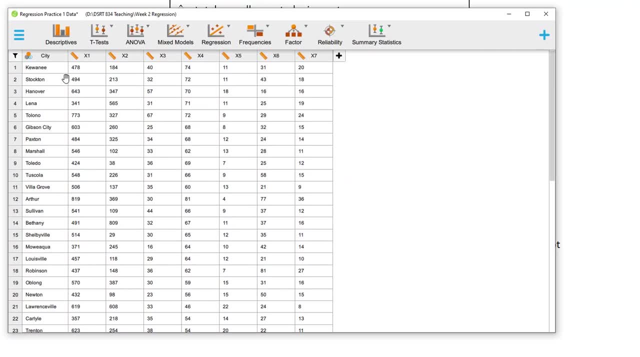 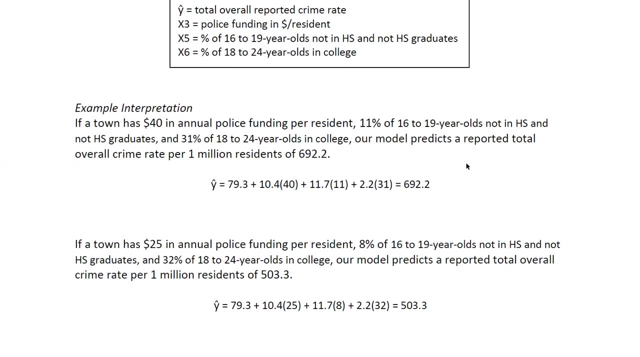 when you take this one. So your estimate minus what you actually get, That's your residual value. You add all of those up, throw it into a beautiful equation if you were doing this by hand- which, yes, back in the old days I have done before, And that's where that R-squared adjusted is going to come from. 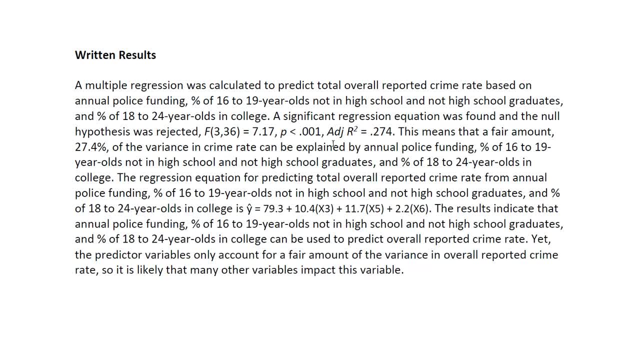 So, moving down to our actual written results, a multiple regression was calculated to predict total overall reported crime rate based on annual police funding percent of 16 to 19-year-olds not in high school And not high school graduates, And 18% of 18 to 24-year-olds in college. That is a mouthful, isn't it?